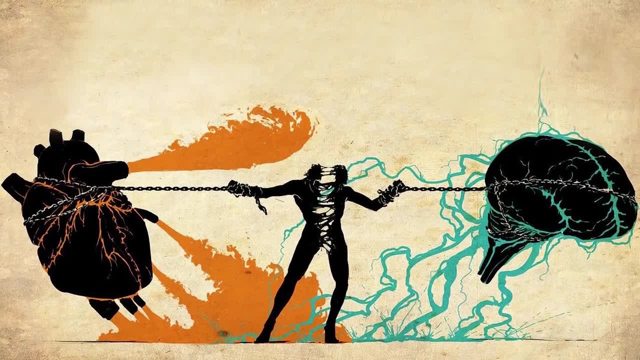 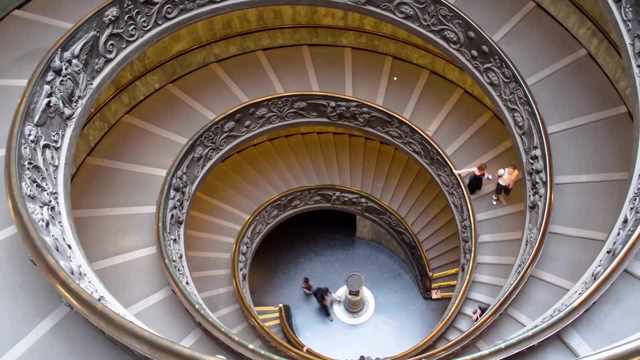 super hardcore. if you hate your classes, you really don't like being a student, then going from your polytech or your community college into a full university is, yes, going to be a step up. going to be a challenge. You're going to struggle, So I would encourage that everyone actually do the full. 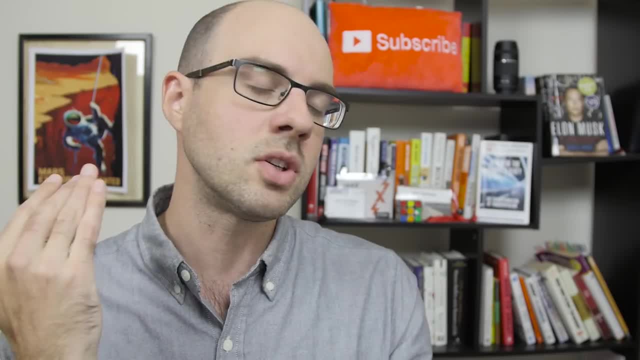 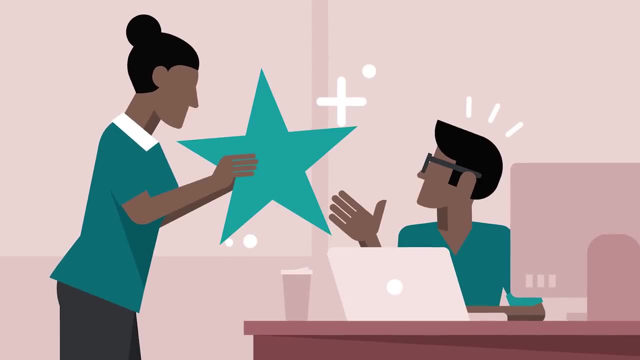 two plus two, unless you're somebody who really hates school and you're just eager to get into the workforce and make a little bit of money, because it's going to be very rewarding to get your four-year engineering degree, and I'm going to explain a little bit more about that right now. So let's talk about, if you were not to go on to the four-year university, what that would mean for you. First of all, you will be constrained to only being an engineering technician for the rest of your career, because unless you have that full engineering degree, you cannot actually call. 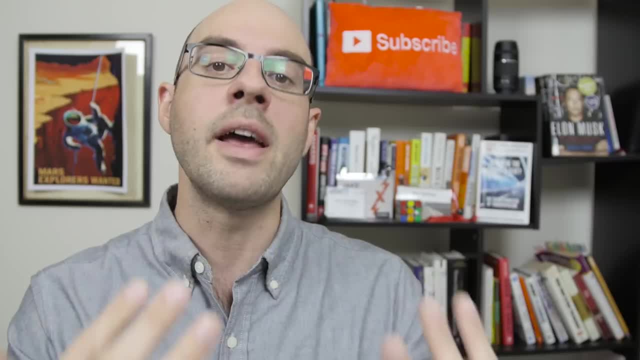 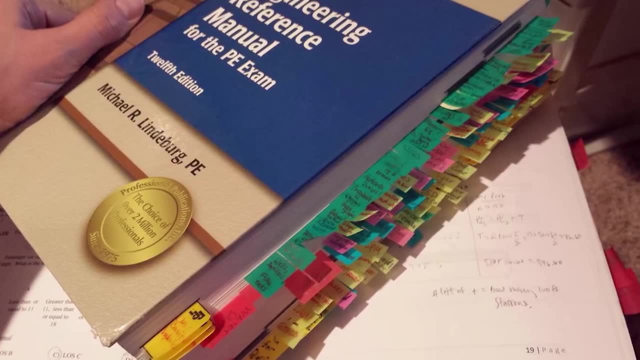 yourself an engineer. You cannot become a professional engineer Here in America. you are not eligible to sit for the PE, the professional engineering exam. You can't stamp stuff, so that means you cannot actually implement design in your work. You most likely will not be able to be a team leader. 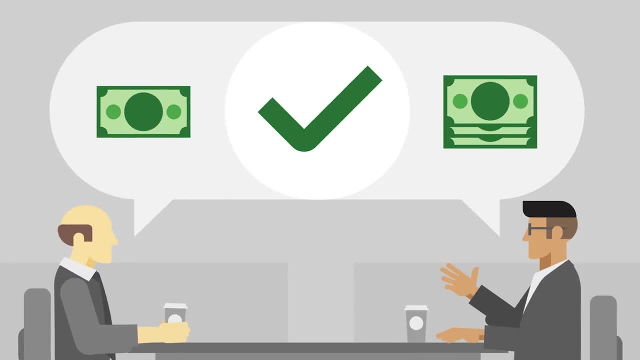 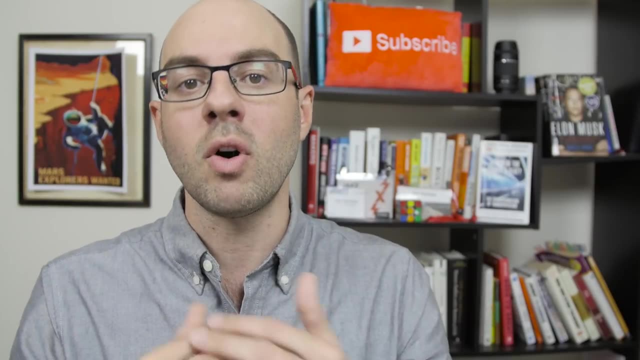 a manager, You will not have a corporate future. You will be limited in the amount of salary that you get, the amount of, say, that you get in the table, because you're just not a full engineer. So in terms of the career, you actually have a whole bunch of disadvantages by not continuing. 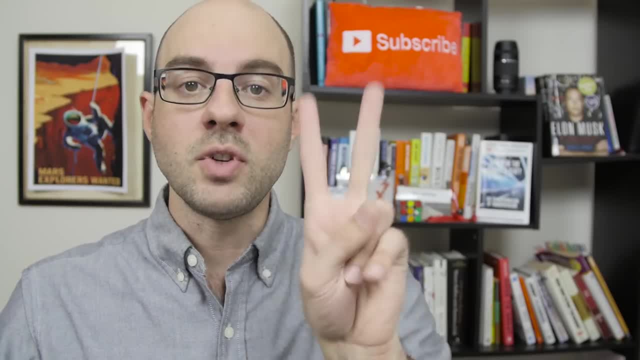 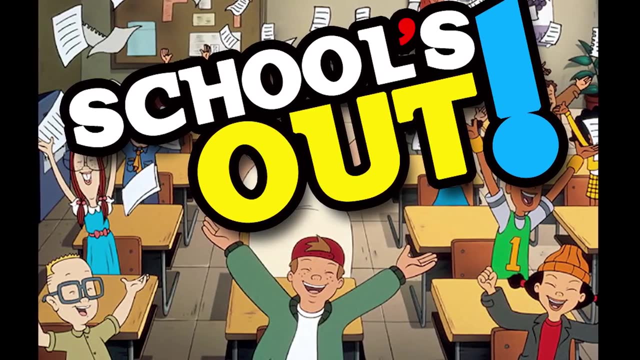 on to getting that four-year degree. What you will find, though, if you just get the two-year technical degree- that, yes, you do two less years of school. you probably have far less debt. It's going to be a little bit easier. You're not going to have the super challenging engineering. 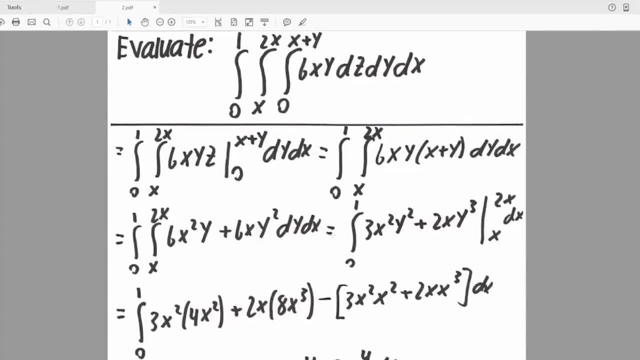 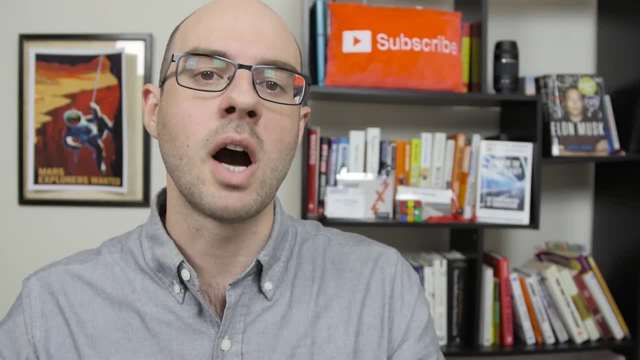 courses in your first two year of that technical school. You're not going to have Calc 3.. You're not going to have Thermo. You're not going to have Dynamics. So, yes, it will be easier, but again, there's lots of career disadvantages with doing this. You have to weigh your options. 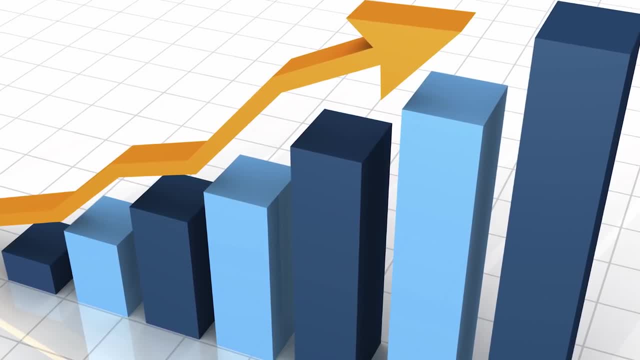 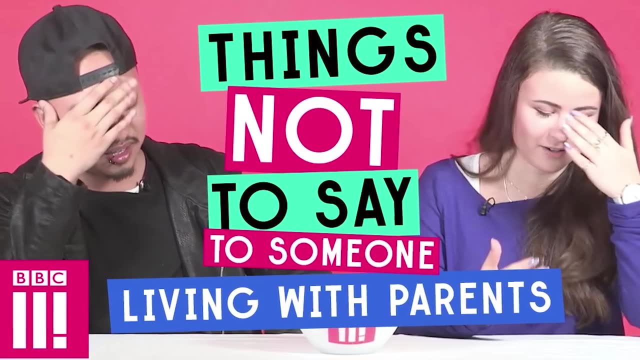 Now there's a whole bunch of advantages of doing the two plus two situation. in general, You've probably saved a bunch of money by not going to the full university for two years. Maybe you can live at home, Maybe you can work on the side. Your grades are probably going to. 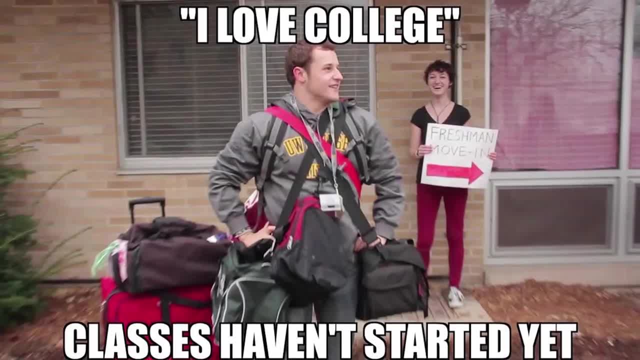 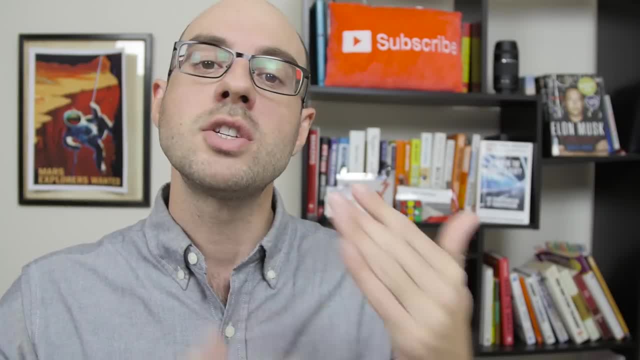 be better in the first two years. You're not going to have that sort of freshmen struggle, that sophomore struggle that a lot of engineers like myself went through. I almost didn't make it through freshman year. I almost didn't make it through sophomore year, So you probably will. 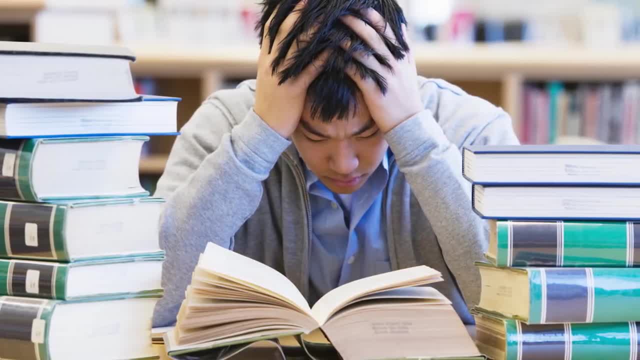 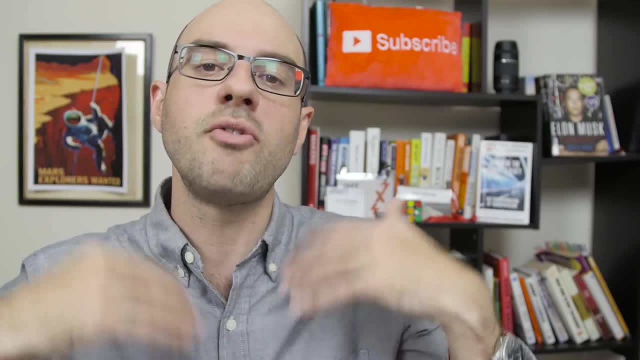 not see that crazy uphill initial front end challenge. But if you transition after two years into that full university there is going to be a learning curve but it gives you the first two years to sort of figure out how to be a student, figure out time management and work ethic and 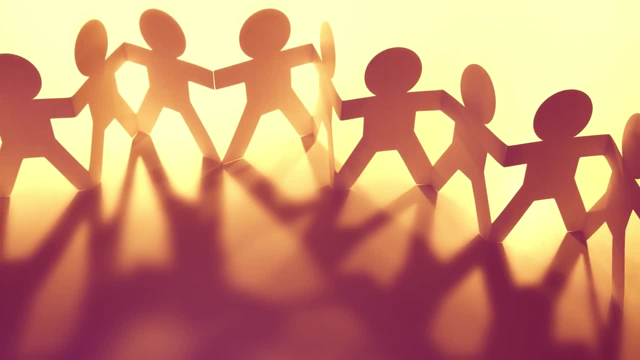 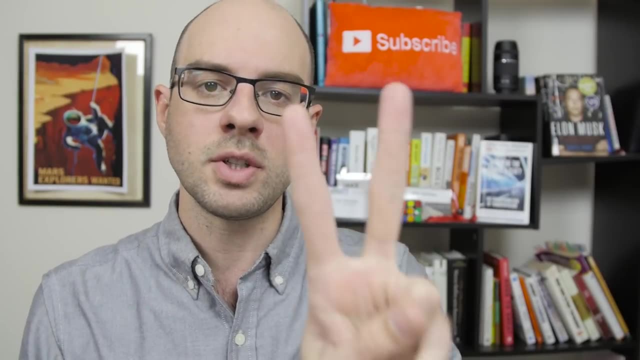 building relationships with your peers and your professors and things like this. So I think you do have a lot of advantages if you decide to go to that full engineering program. So, if you choose to become a technician, if you choose to only do the two years, 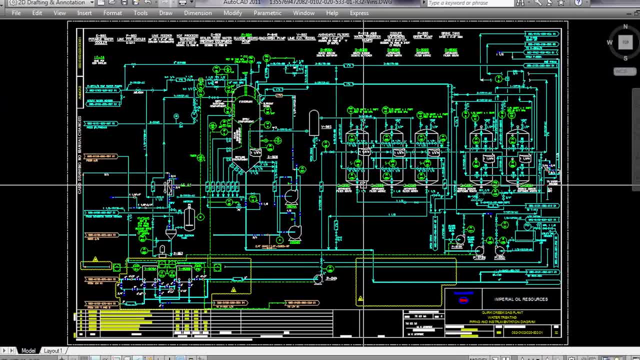 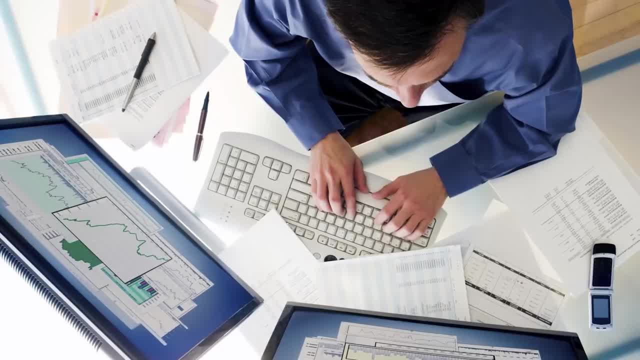 what that means for your career is: you will probably become a drafter, You'll probably be a support technician. You'll do calculations, you'll do estimates, you'll do drawings, you'll do figures and exhibits. You'll probably do data entry. 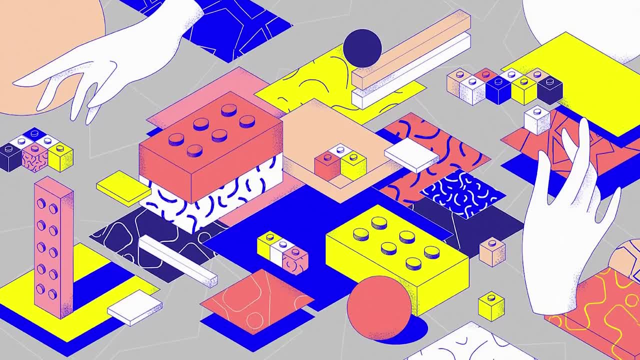 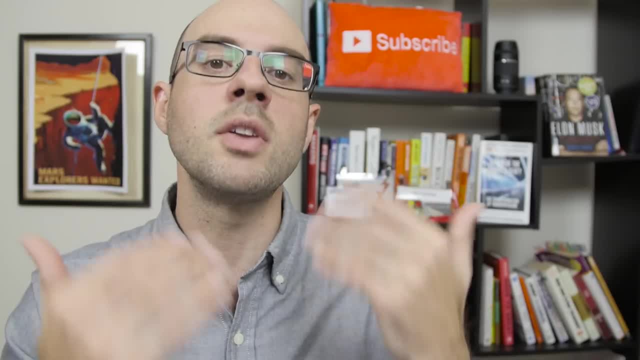 maybe some data analysis, But again, you will never actually be able to participate in design. You'll definitely not be a team leader and you will do the heavy lifting, what they might call grunt work. That's what your career, that's what your future is destined to be. So, if you like, 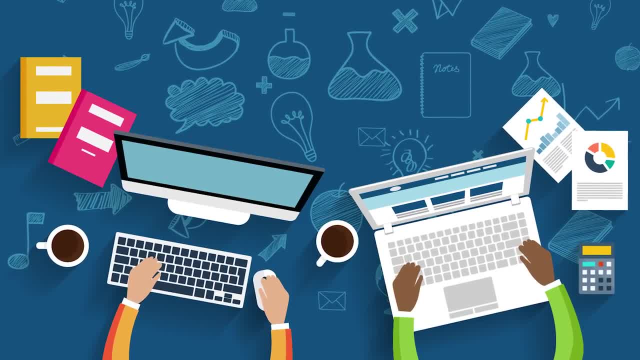 that sort of stuff, great. If you want to get paid less, if you don't want to be a leader, if you're just eager to work, maybe you just hate, hate, hate being a student. Maybe this is for you. 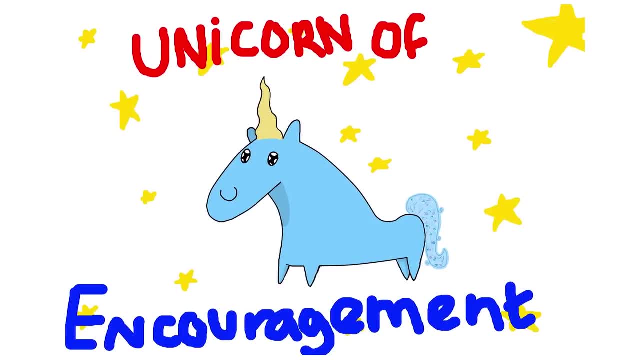 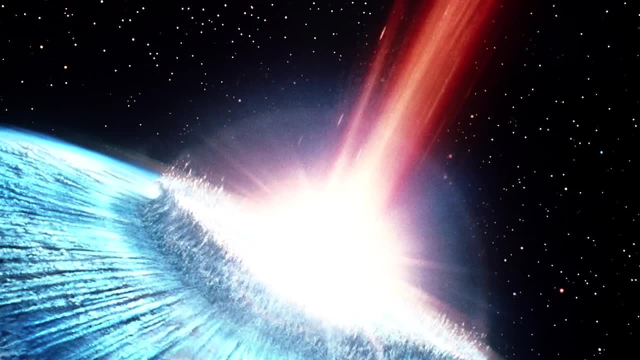 I'm going to highly encourage you guys to continue on and do the two plus two. get that four year degree. Being an engineer is respectful. It's prestigious. We have an impact on society. You're going to be able to feel good about your career. You're going to be able to make a difference. 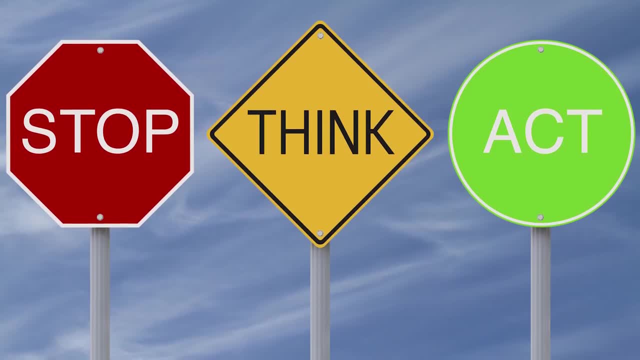 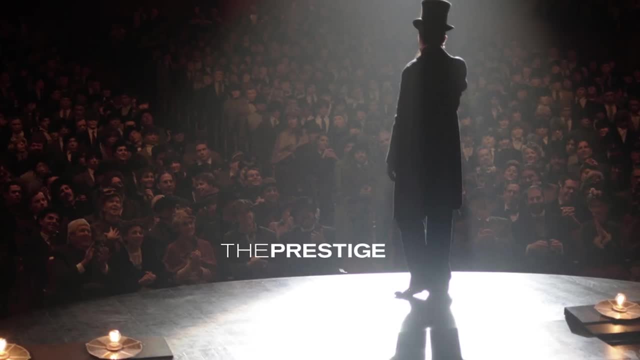 You're going to be able to design things, make stuff safer, make things more efficient, create scenarios where they can save money. You're going to make more money than average. engineering is prestigious. There's a reason why we honor doctors and lawyers and engineers. 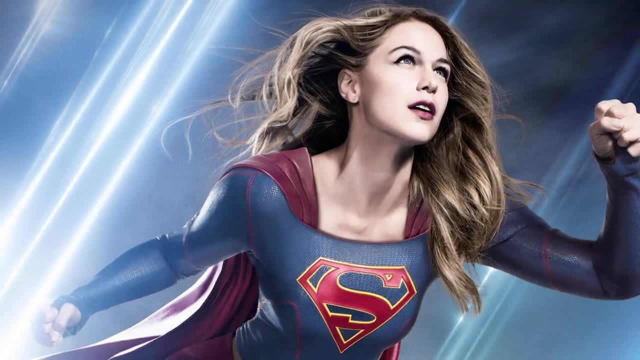 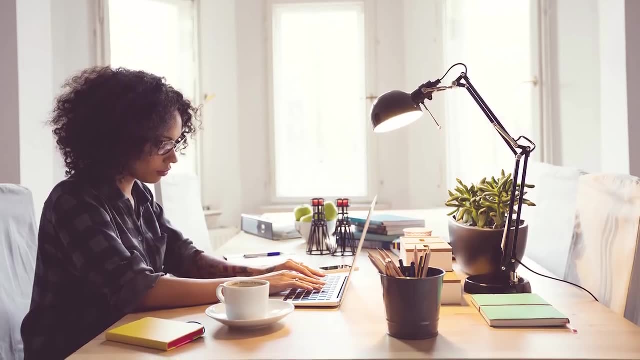 is because we do have an impact, We are respected. So there's lots of advantages of just becoming an engineer and there's even more baked in advantages that you don't realize until you're working, until you see the stuff in the world. But if you have an engineering degree you can even change careers and it's probably going to be okay. 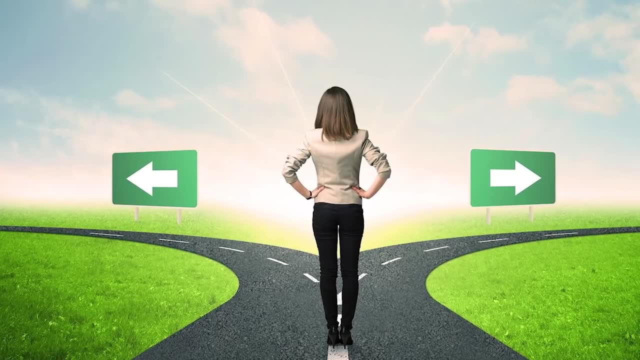 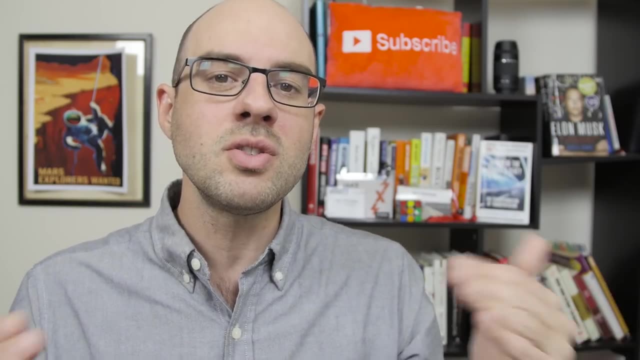 because most people know that you're going to be able to figure out whatever you want. You're an engineer. It almost brands you with this stamp of respect. So if you want to go back to grad school, no matter what avenue you choose, you're going to be able to get into those programs. Again, if you want to switch up your career, you're going to be able to get a job, even if you leave engineering. you're going to be fine with that engineering degree. Oppositely, with an engineering technician diploma, you're not going to be able to work anywhere. 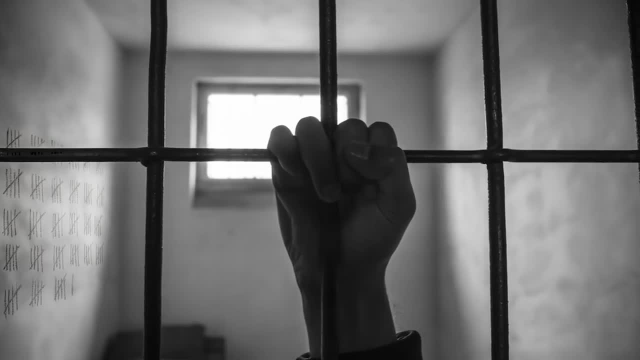 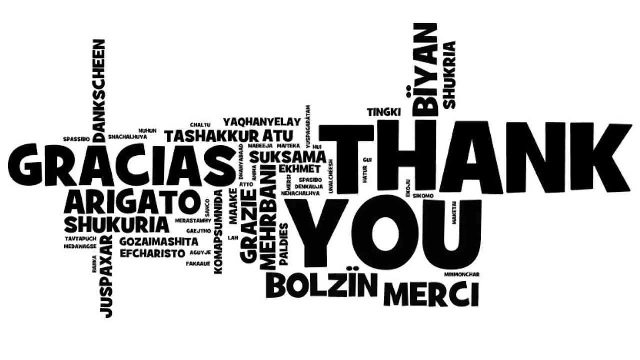 You're not going to have enough respect and authority to just throw your resume around and get picked up by a company. You don't have that option. So, though, again, thank you for the awesome question. If you have more concerns or little micro questions within this conversation, please make sure you tell Brian. comment on this video.